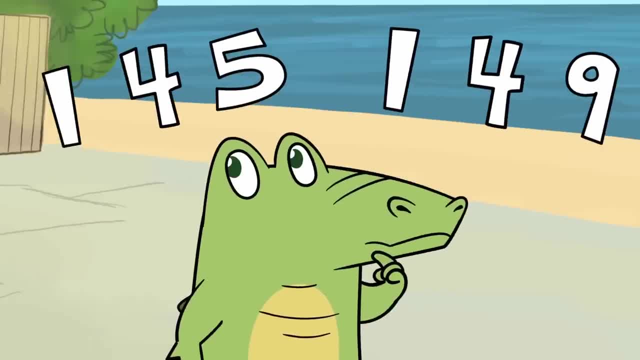 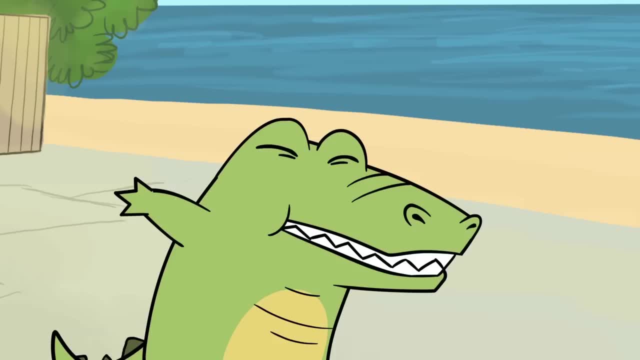 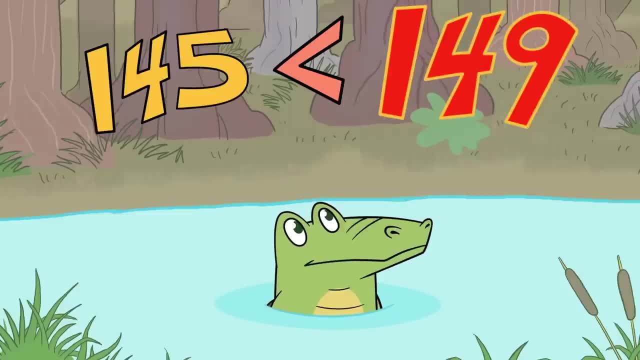 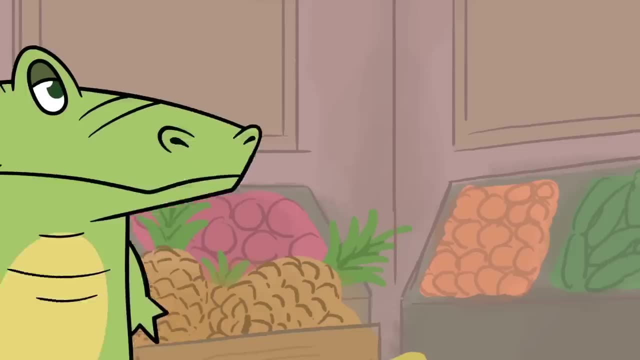 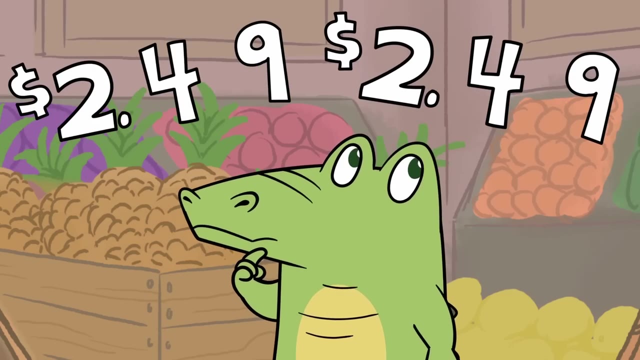 It's the number that is greater. The number that is least is never part of its speech. Now, the numbers are the same on both sides. The gator wants to eat, but he can't decide. Neither is greater or less. it's a perfect tie. So the alligator writes an equal sign. 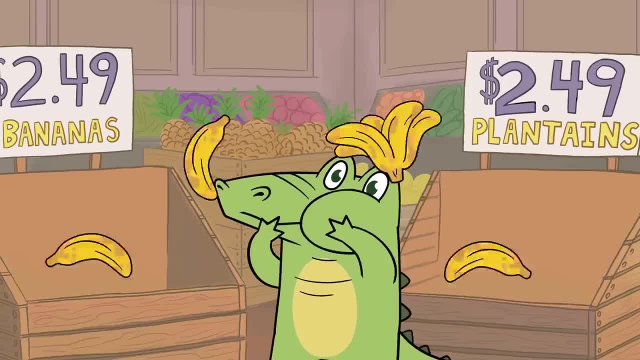 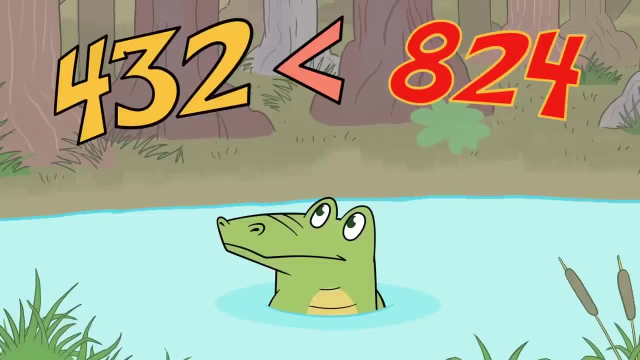 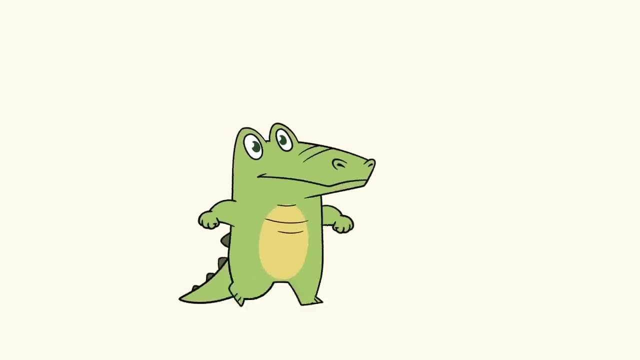 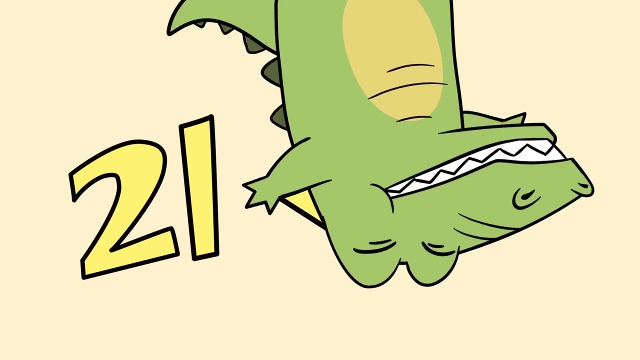 The hungry alligator is the number that is greater. The number that is least is never part of its speech. The hungry alligator is the number that is greater. The number that is least is never part of its speech. If there's a line underneath the greater than 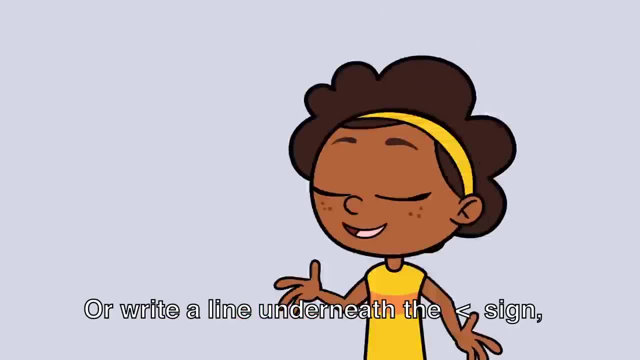 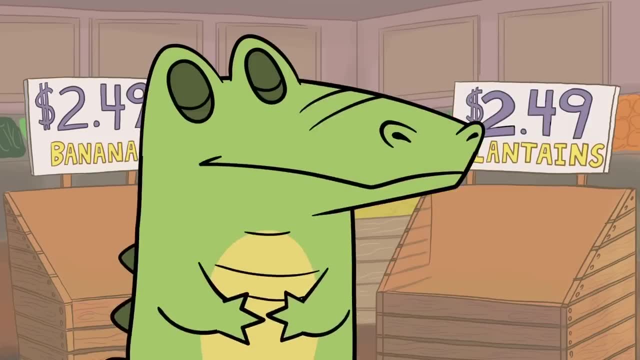 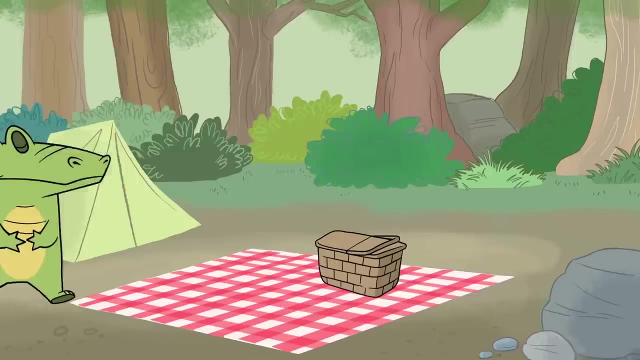 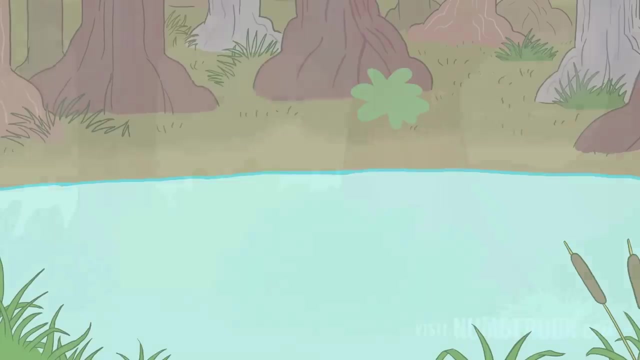 sign. greater than or equal to is how the sign is defined. I'll write a line underneath the less than sign, And less than or equal to is the name of the design. Hi there, I'm an alligator, so let's keep this snappy. 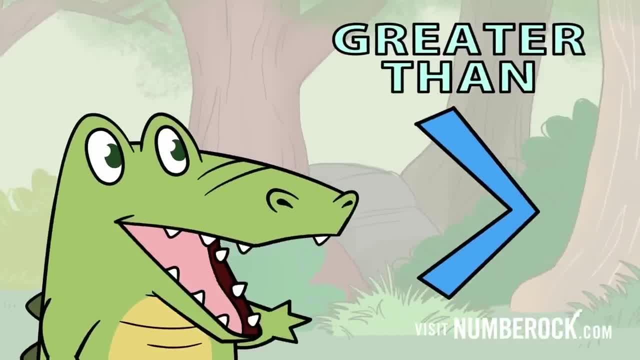 I'm an alligator, so let's keep this snappy. I'm an alligator, so let's keep this snappy. I'd like to take this opportunity to tell you that the greater than symbol goes from big to small, And it's called the greater than symbol.